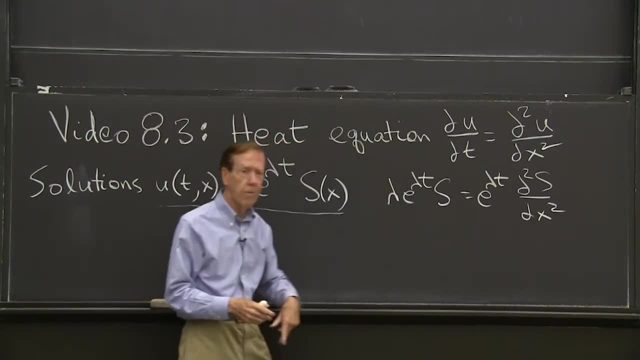 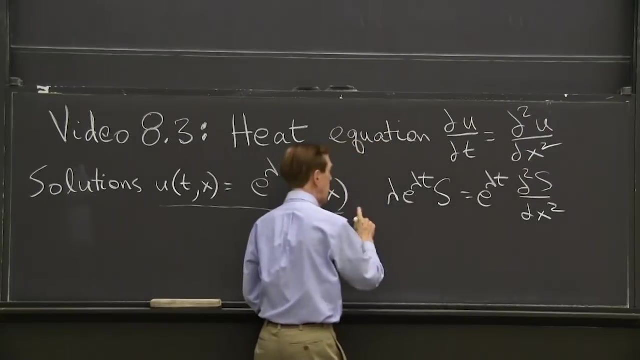 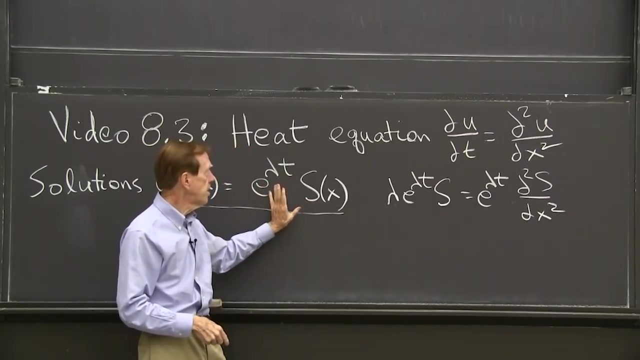 And, just as always, I substitute that into the differential equation to discover what determines s s of x. OK, the time derivative brings down the lambda. The space derivative has two space derivatives, So that's what I get when I substitute e to the lambda t s. 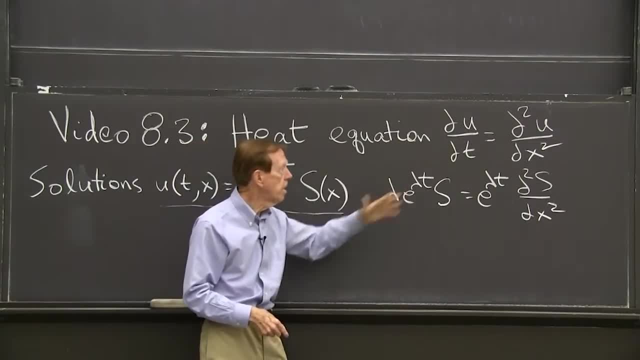 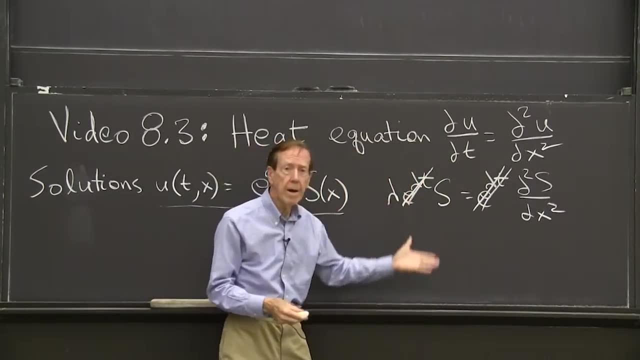 eigenvalue times eigenfunction into the equation, And always I cancel e to the lambda t- That's the beauty of it. And I have an eigenvalue equation Or an eigen, and I'm looking again for a function. So 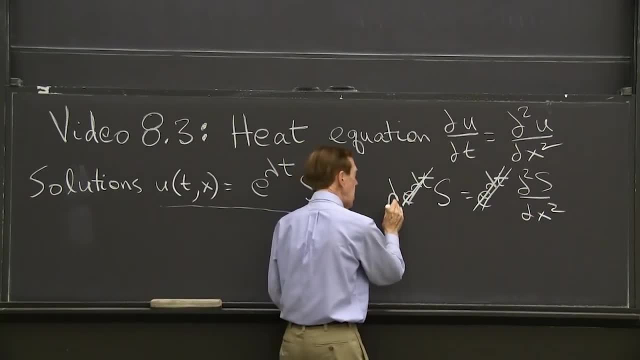 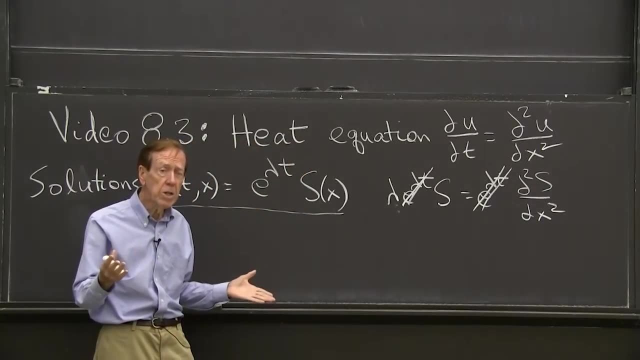 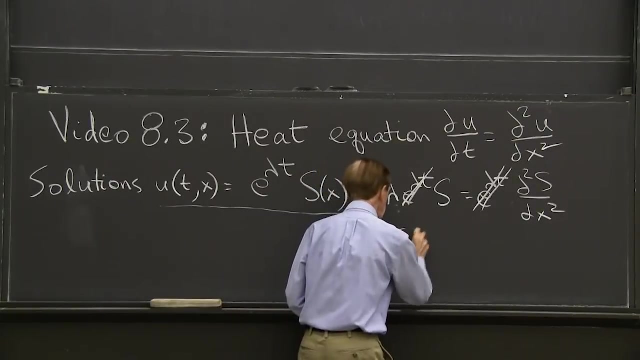 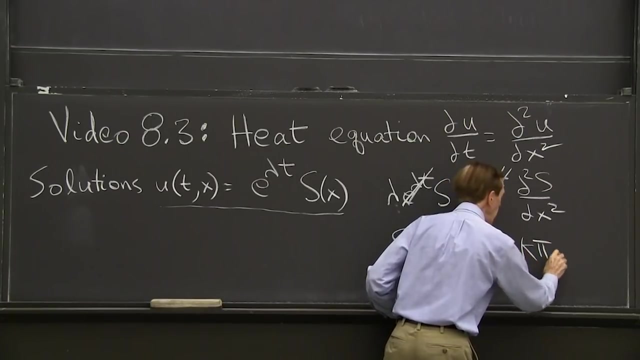 So the second derivative of my function is lambda, some number times my function. OK, What I'm looking for? functions s there'll be sine. functions s will be s of x will be the sine of k, pi, x The sine of x. 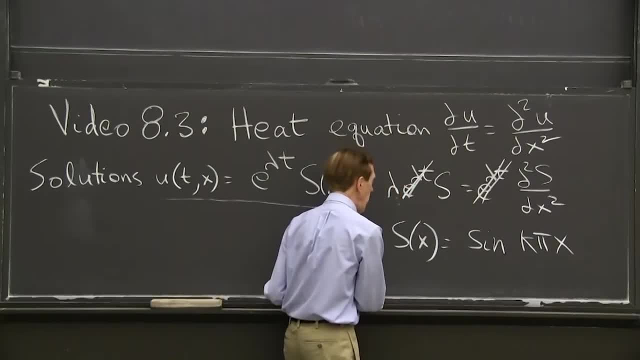 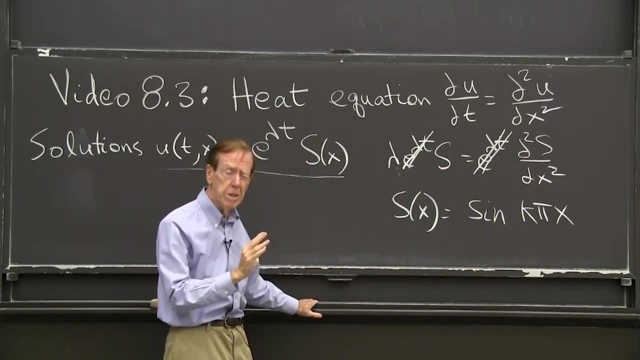 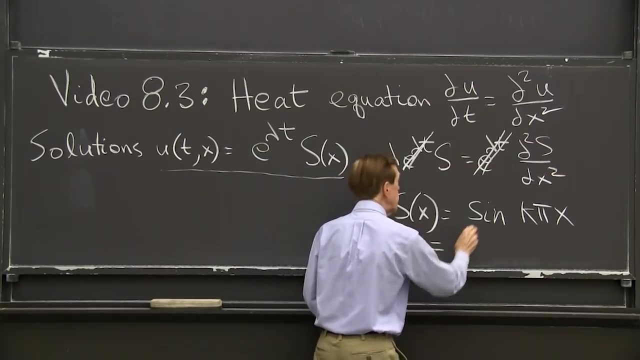 The sine of something times x, What's the eigenvalue? Take two derivatives of this. I get back sine k, pi x, which is so? that's great, It's an eigenfunction, And out comes the eigenvalue. lambda is well. 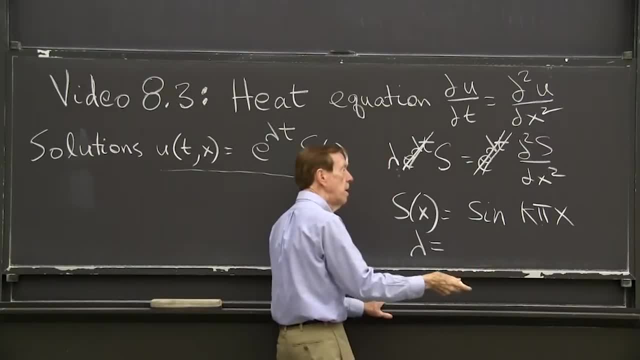 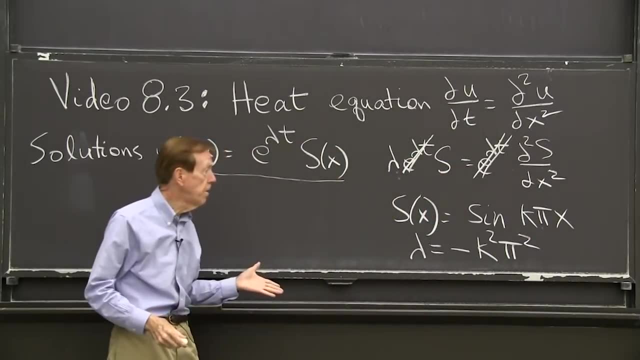 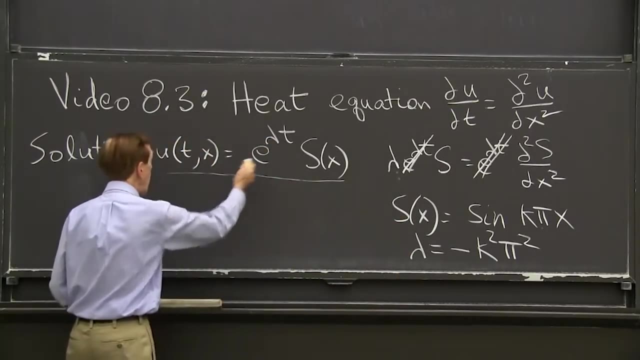 when I take two derivatives, k, pi comes out twice with a minus sign. So it's minus k squared, pi squared. So I have found a bunch of eigenvalues, The eigenvectors, eigenfunctions and the eigenvalues. So now, so this was a simple pair. 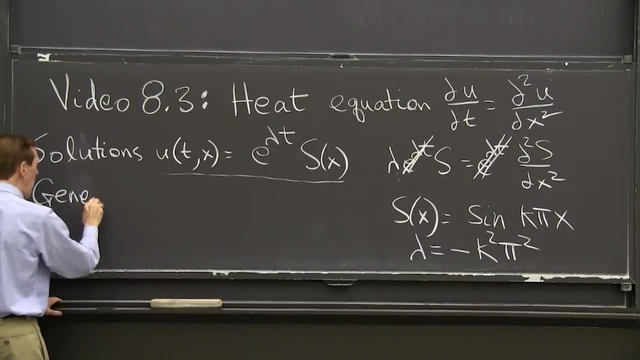 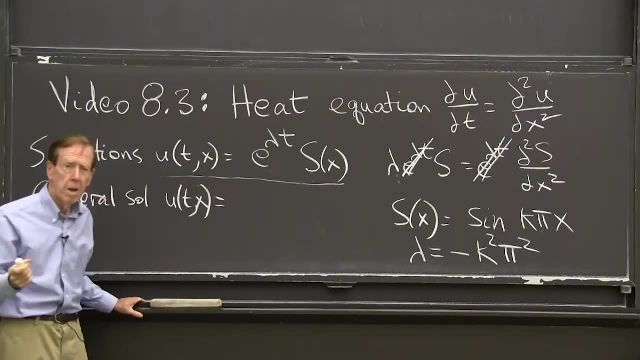 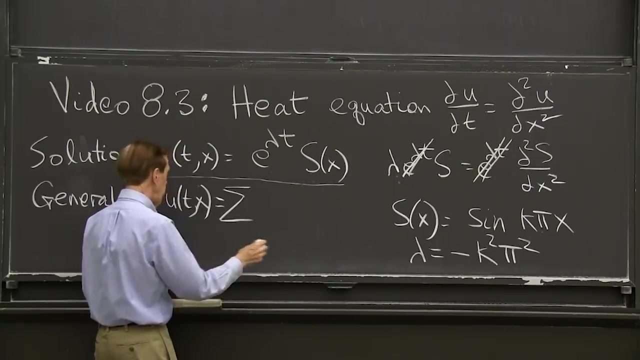 But now general solution. the general solution u of t x will be: if I know several solutions and I have a linear equation, I just take combinations. That's always our way: Take combinations of those basic solutions. So I'll have a sum k going from 1 to infinity. 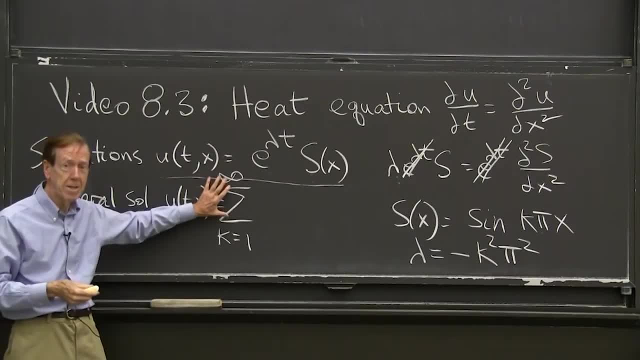 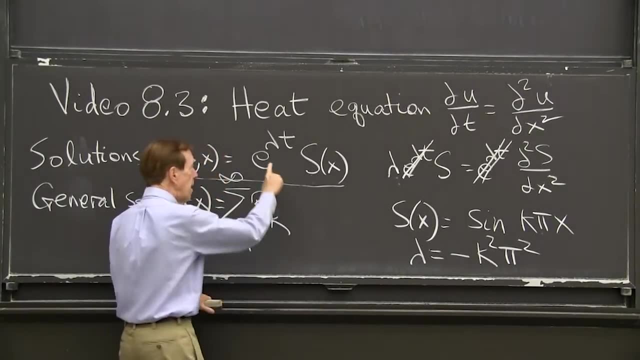 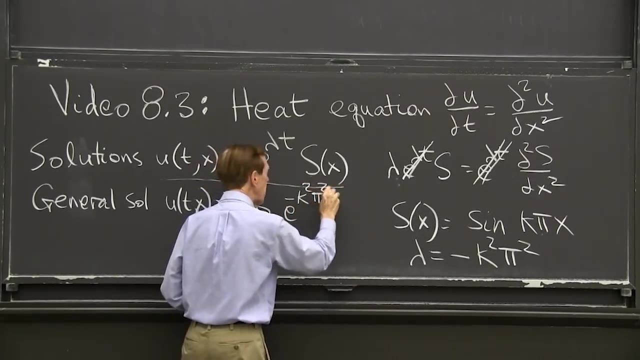 In partial differential equations. I need a big sum here of some coefficients. Let me call them bk times. this solution e to the lambda What was lambda Minus k squared pi squared t times s s number k. I should have given that. 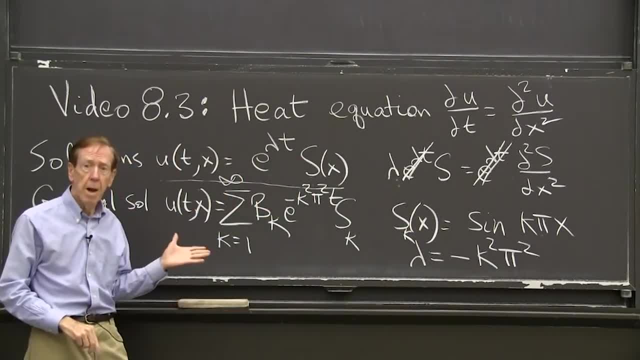 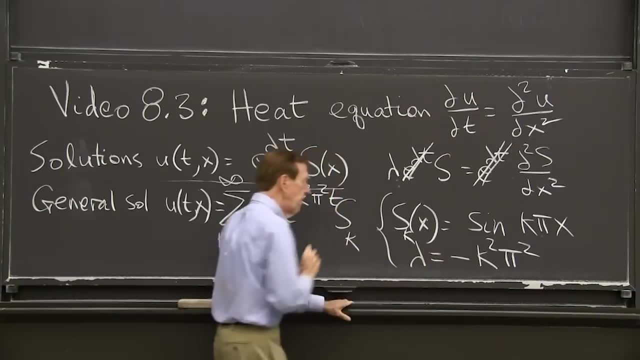 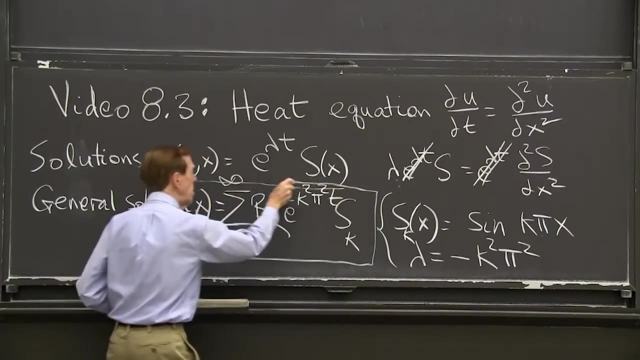 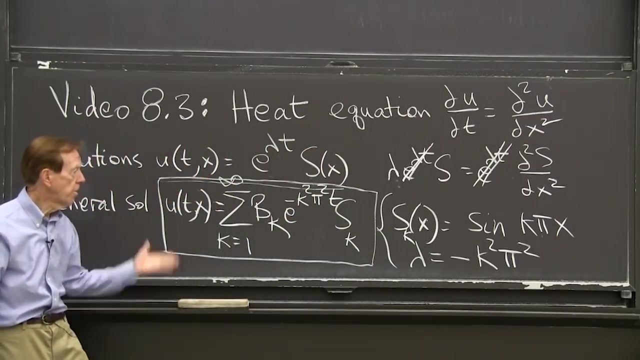 And this eigenfunction it's a number k. So this is my family of eigenfunctions and eigenvalues, And then this is the combination of these solutions. There's the general solution And for sk I should have written in sine: k, pi x. 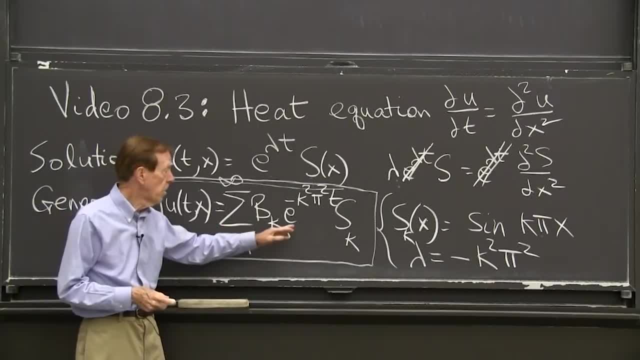 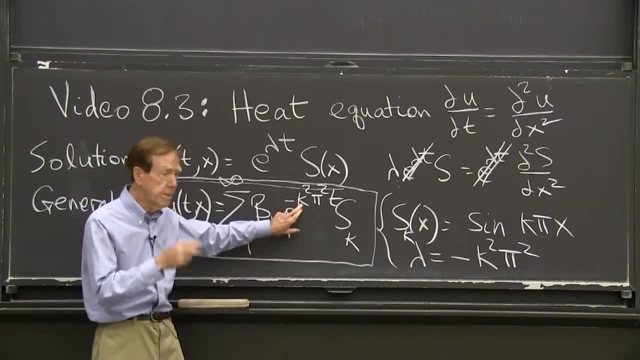 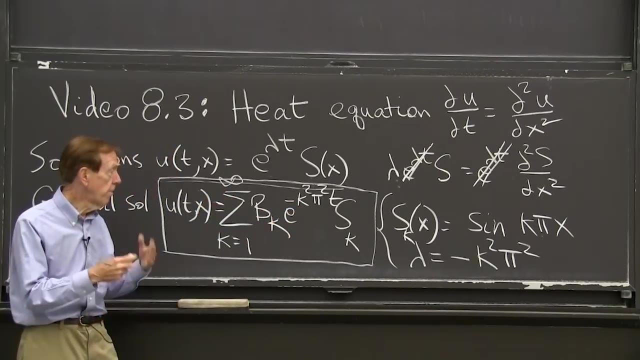 So that's the dependence on t. Let's have a look at this. So the dependence on t, Dependence on t, is fast decay, And as k gets larger, later terms in this sum the decay is really fast. So the term that decays most slowly, k equal 1,. 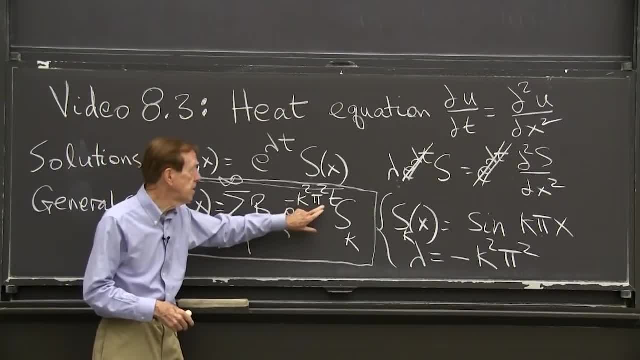 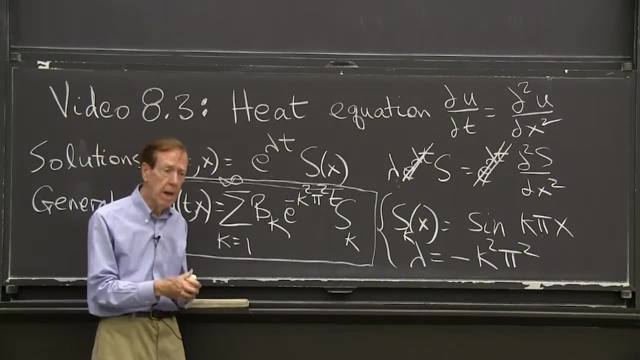 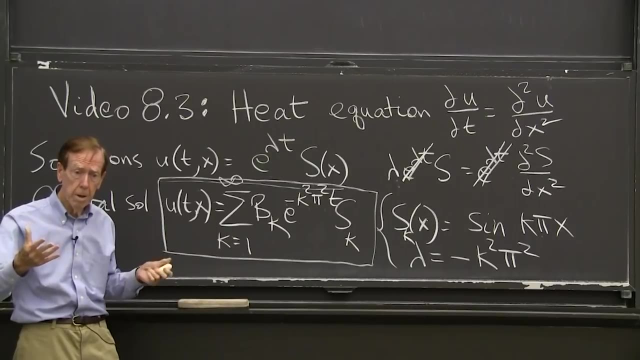 there'll be a b1 and e to the minus pi squared t. That's decaying already pretty fast. When I'm talking about decay, what's happening here? I have a bar, a material bar. The ends of the bar are kept at temperature zero. 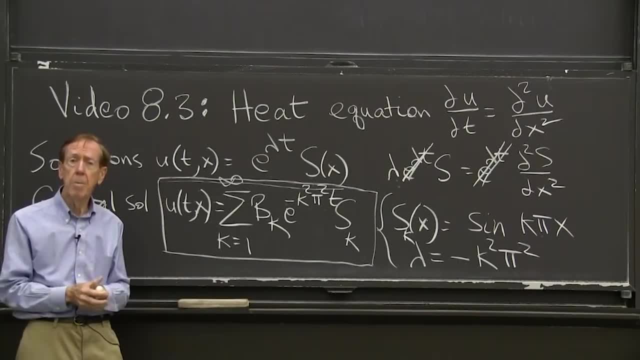 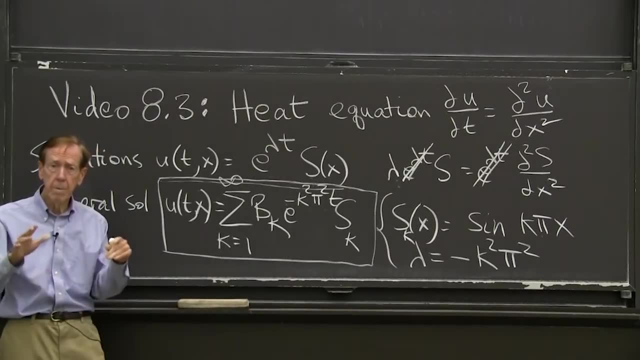 They're frozen And heat is in the bar. Heat is flowing around in the bar And where is it going? It's flowing out the ends. The bar is approaching freezing, Freezing, Freezing. The ends are kept at freezing. 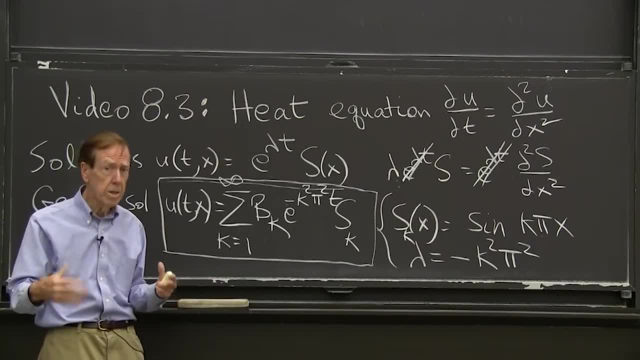 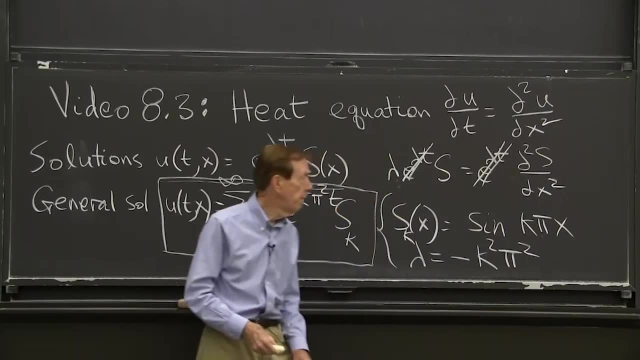 And the inside of the bar, whatever heat is there at the beginning is going to flow out the ends. So you see that I have these sine functions When x is 0, the sine is 0. So that's frozen at one end. 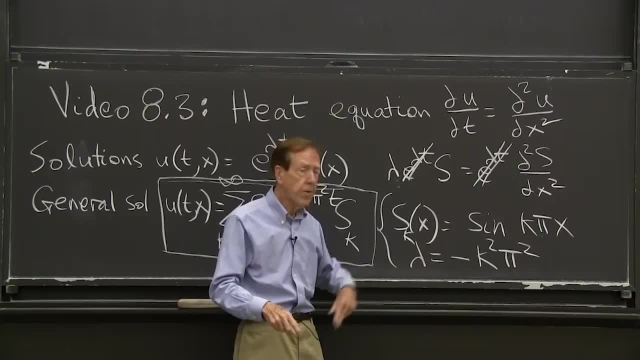 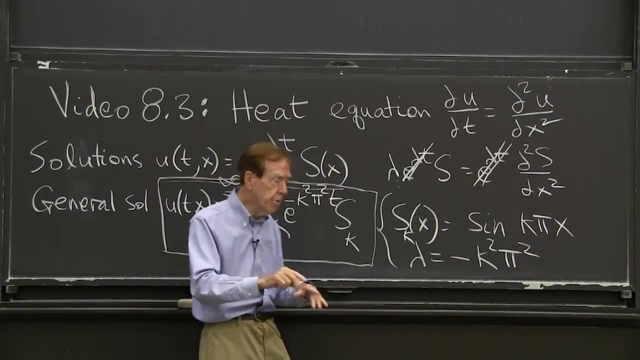 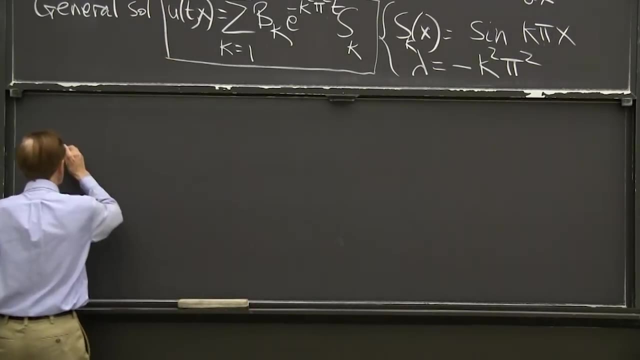 When x is 1, I have the sine of k, pi, which is again 0. So it's frozen at the other end. So I'm freezing it at both ends. The temperature is escaping out of the center. So let me graph the solution. 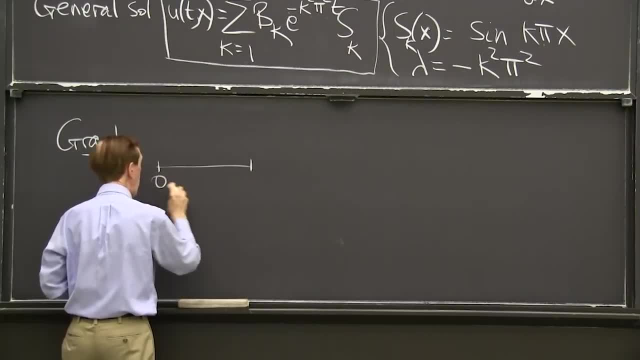 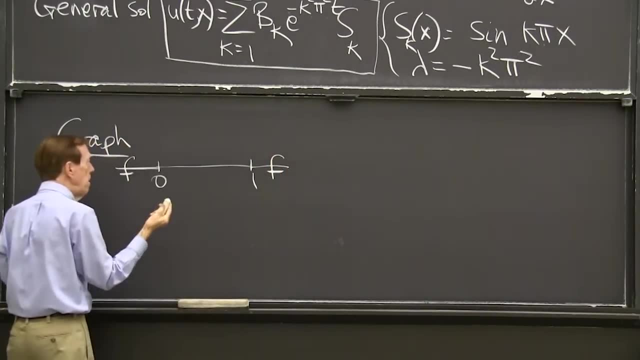 So maybe I start with. here's my bar, from 0 to 1.. And I'm keeping it frozen F for frozen, F for frozen. at that end, Maybe I start off with a warm bar. So u at 0.. u at 0.. 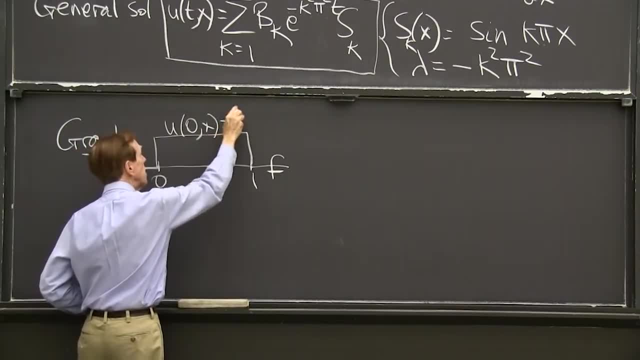 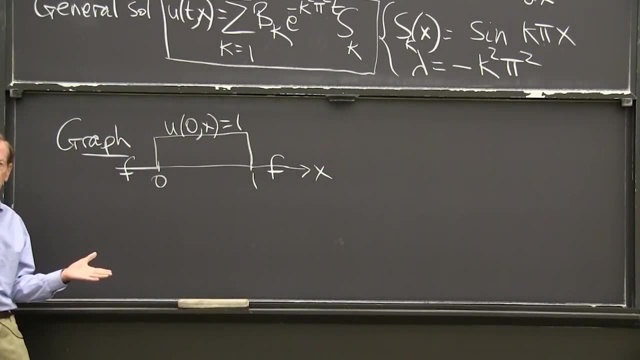 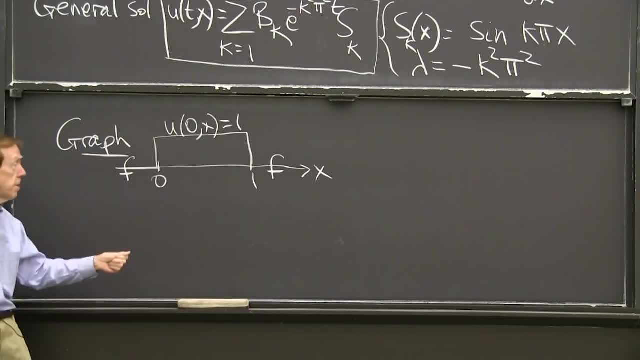 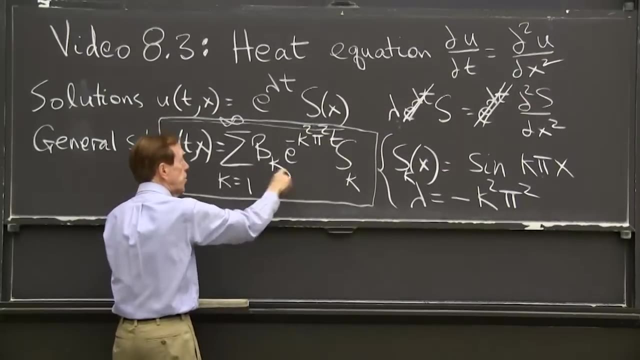 So the heat is escaping out the two ends Out the end x equals 0. And out the end x equals 1.. And the solution will be this: Let me remember what the general solution looked like, And I have to find these numbers. 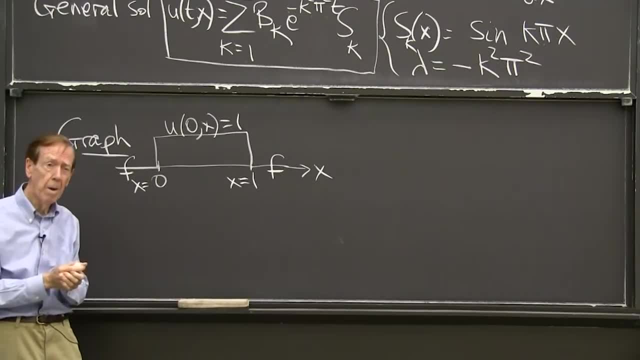 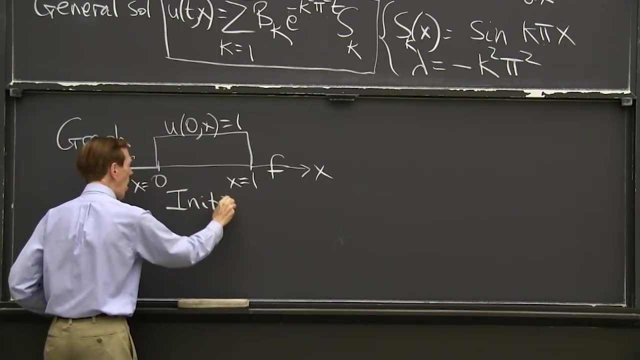 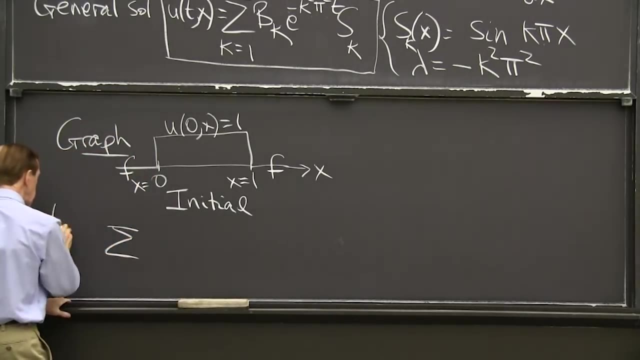 And those numbers. of course, the numbers are always found by matching the initial conditions. This is the initial, This is the initial picture, So I have to match that by. so this is t equals 0.. I have to match that. 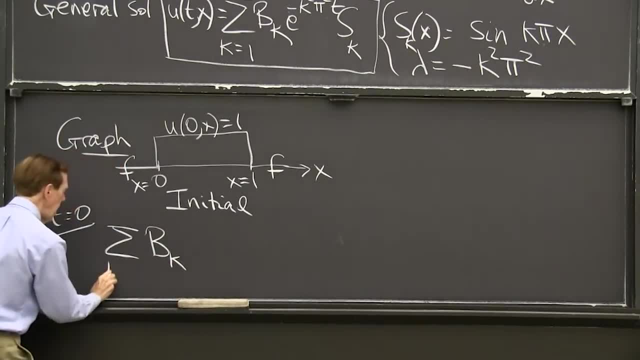 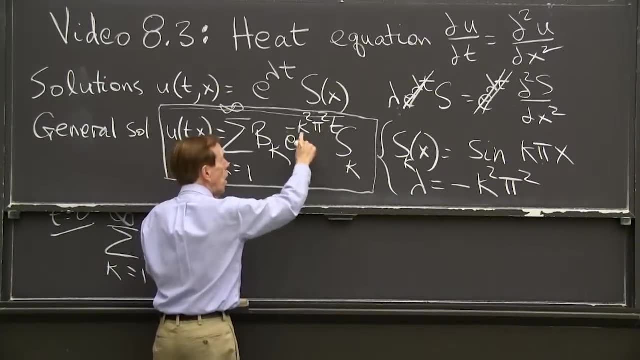 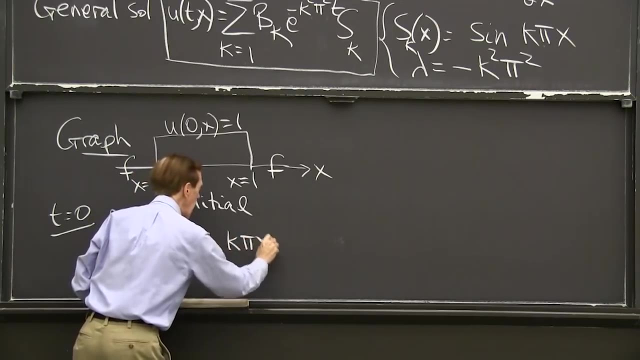 So this is: t equals 0. I have to match the sum of bk. This is k, going from 1 to infinity. When t is 0, this is 1.. And I just have the sk, the sine of k, pi, x. 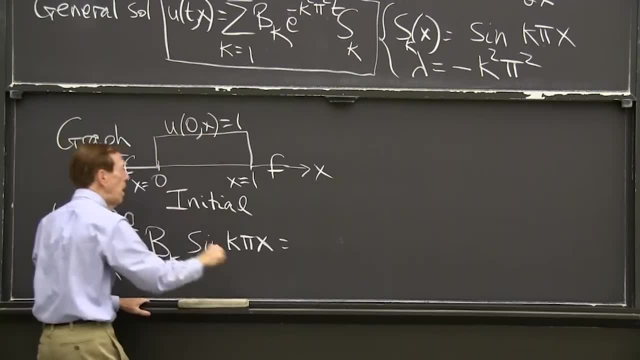 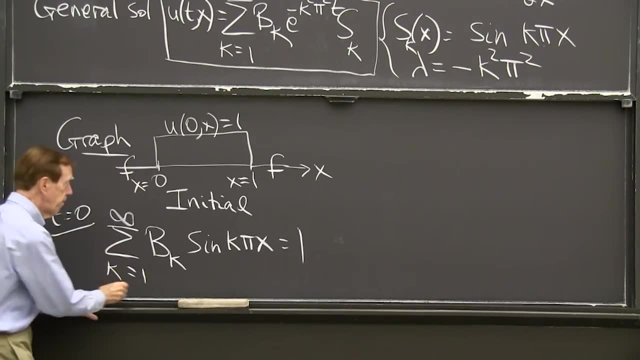 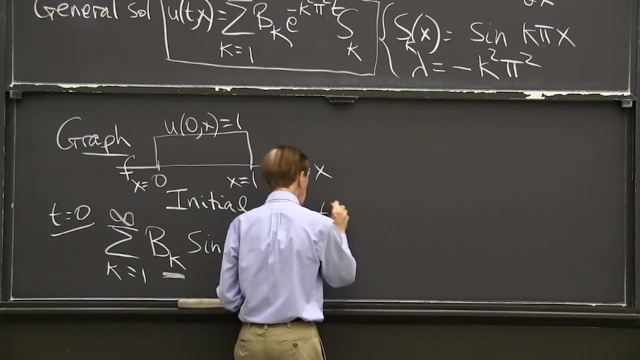 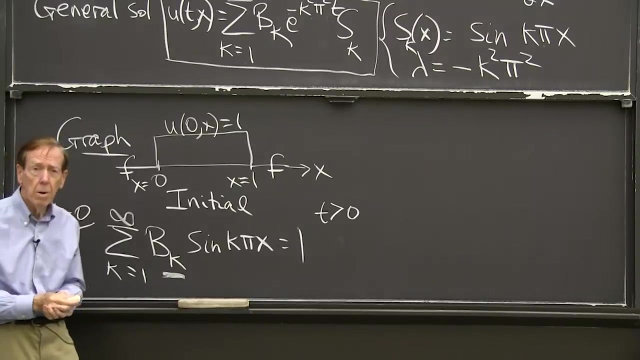 That has to match the 1. And when I from that I find the bk And then the final solution: t greater than 0, uses those bk's And we're again faced with a Fourier series problem. Any time I have to find these coefficients. 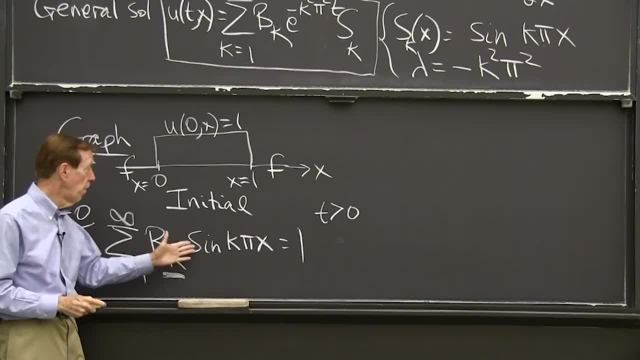 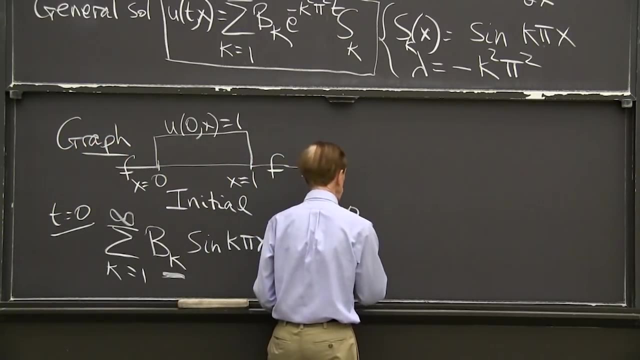 this is a Fourier sine series. I have only sines, not cosines here, And I'm finding the coefficients So that this will match 1,, the initial condition, And then for t greater than 0, the solution. u will be: 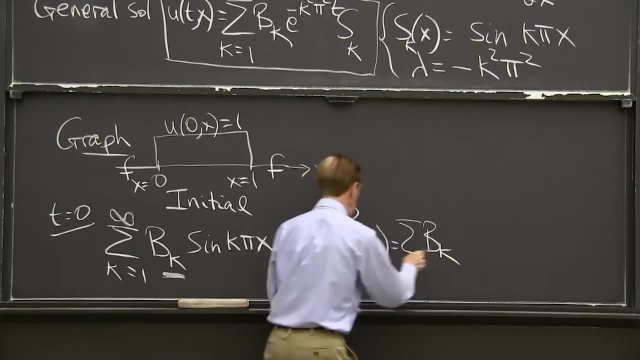 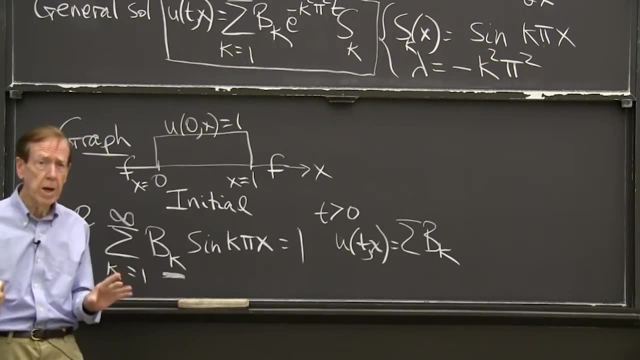 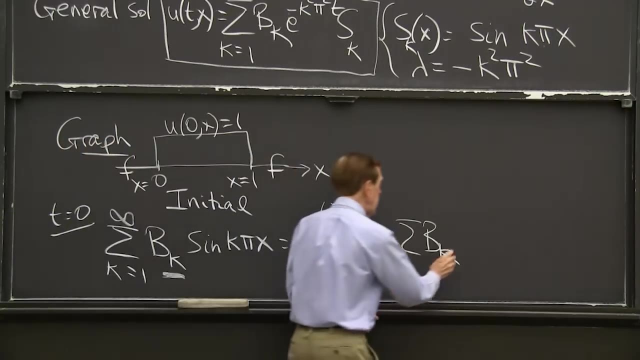 as we said, the sum of these bk's, which come from the initial conditions, come from this Fourier coefficients. We still have to do that video on Fourier series to know what these numbers will come out to be. times the e to the minus, k squared, pi squared.